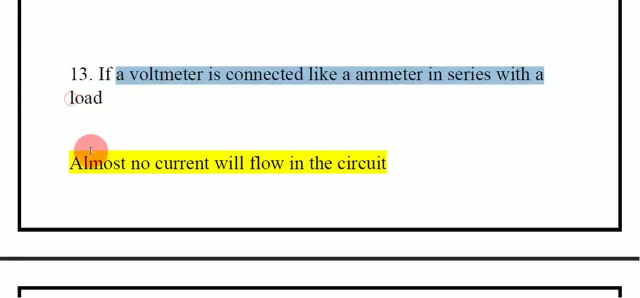 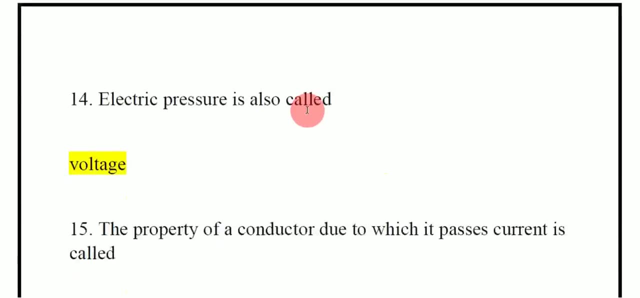 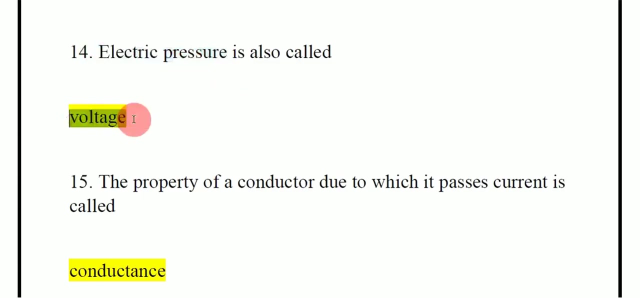 connected like a emitter in a series with a load, almost no current will flow in the circuit. so remember, if a voltmeter is connected like a emitter in a series with a load, almost no current will flow in the circuit. electric pressure is also called voltage. okay, electric pressure is also called voltage. the property of conductor due to 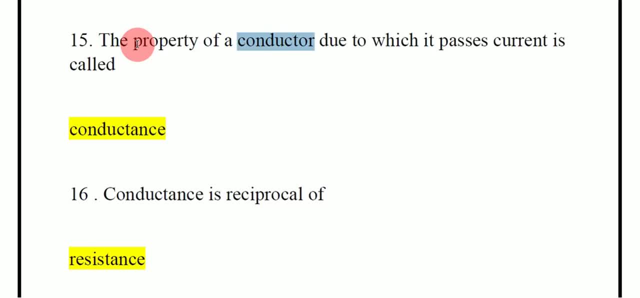 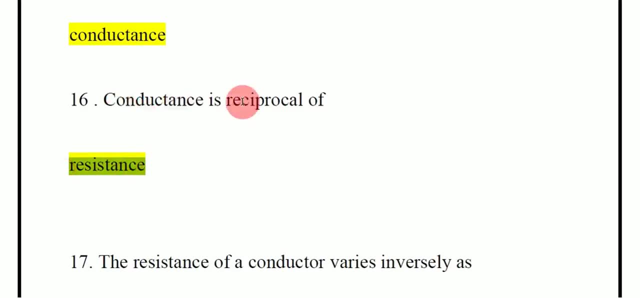 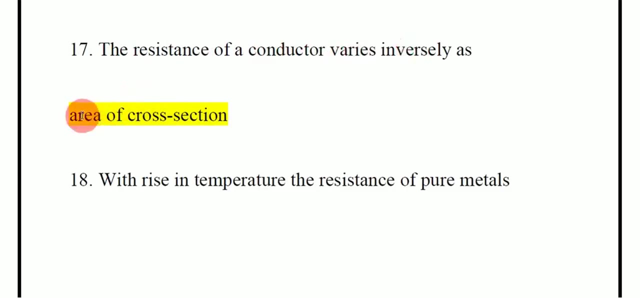 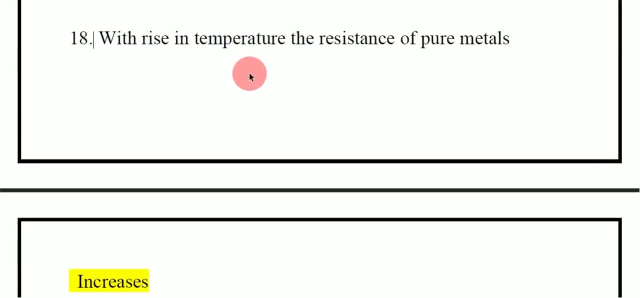 which it pass current. so this type of property is known as a conductance. conductance is a reciprocal of resistance. okay, Okay, conductance is a reciprocal of resistance. The resistance of conductor varies inversely as area of cross section. With rise in temperature, the resistance of pure metal increase. 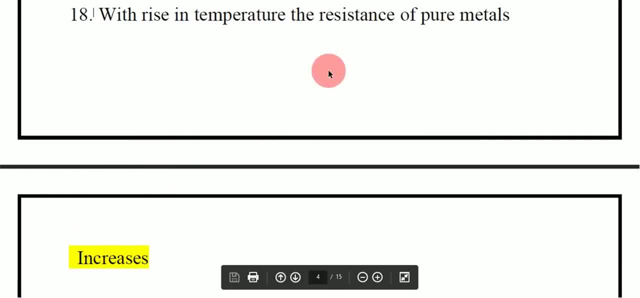 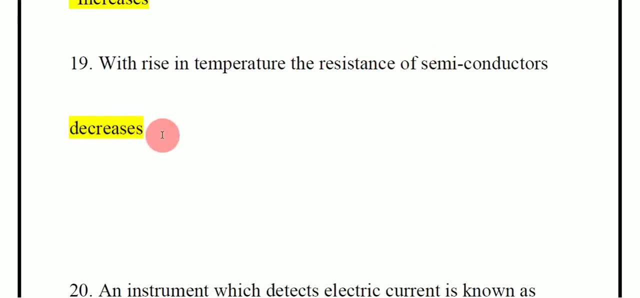 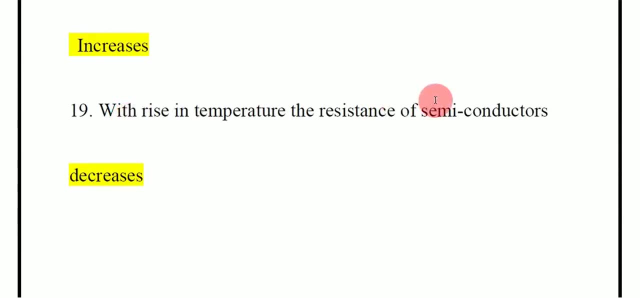 Okay, with rise in temperature, the resistance of pure metal increase. With rise in temperature, the resistance of semiconductor decrease. Okay, so remember: the rise in temperature, the resistance of pure metal increase, but semiconductor the temperature. when rise in temperature, resistance of semiconductor will be. 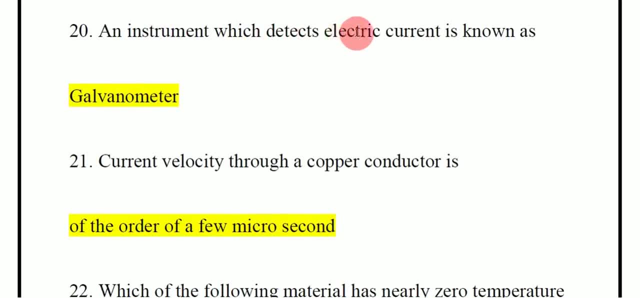 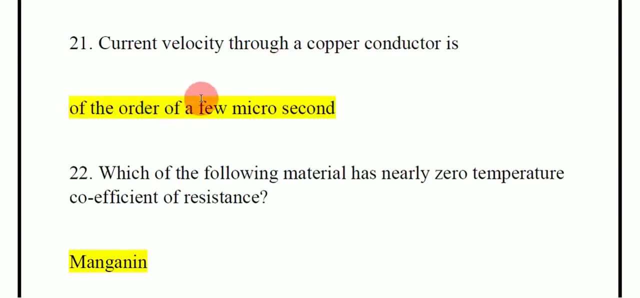 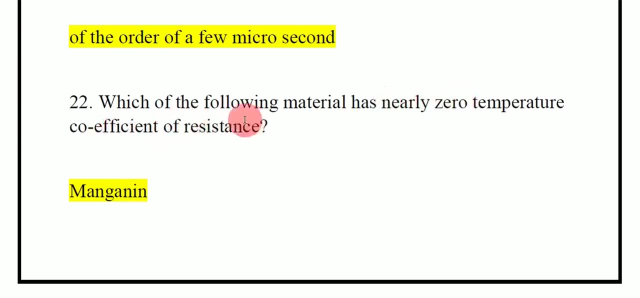 decrease An instrument which detects electric current, so that is galvanometer. Current velocity through a copper conductor is of the order of few microsecond. Which of the following material has nearly zero temperature Coefficient of resistance? so manganese. manganese has a zero temperature coefficient of resistance. 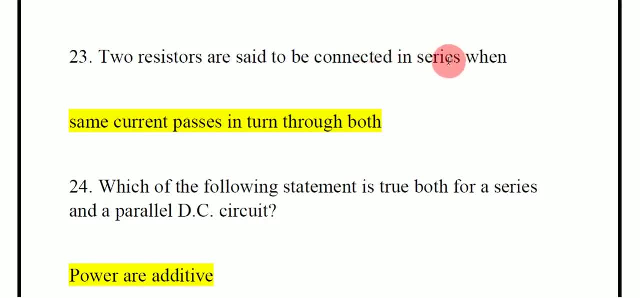 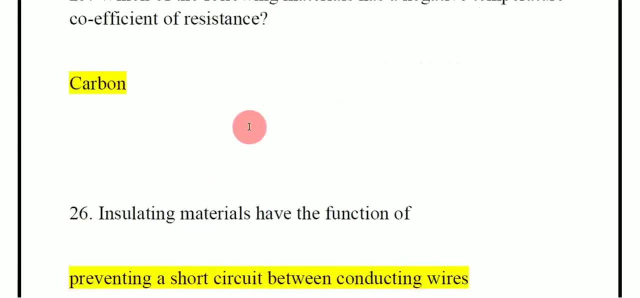 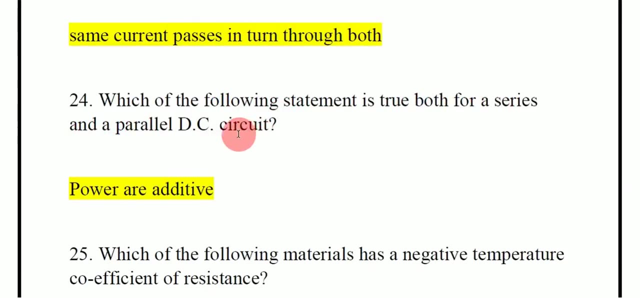 Two resistors are said to be connected in series When same current pass in turn through both. Okay, now, which of the following statement is true both for a series and parallel DC circuit. So power are additive, So this is the true power. 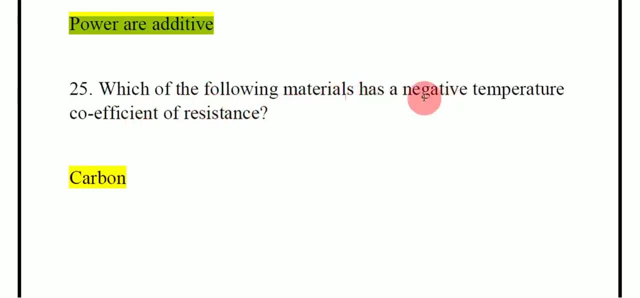 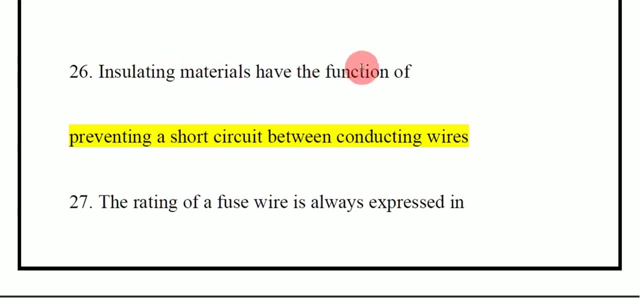 Power are additive. Which of the following material has a negative temperature coefficient of resistance? Negative temperature coefficient of resistance. so carbon, Carbon, has a negative temperature coefficient of resistance. Insulating material have the function of preventing a short circuit between conducting wires, So we are using insulating materials. 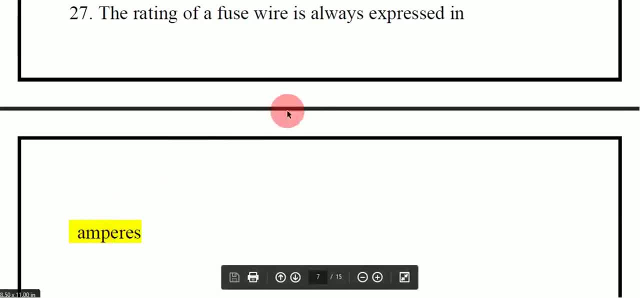 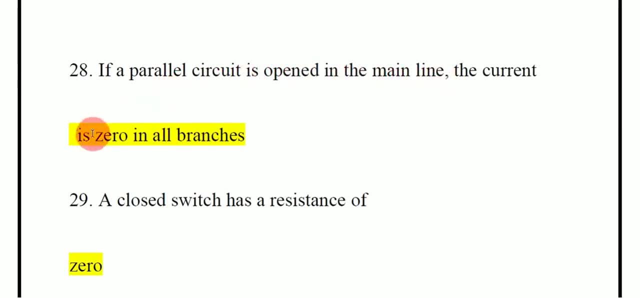 The rating of fuse wire is always expressed in a MP. Okay, if a parallel circuit is opened in the main line, the current is zero in all branches. So remember, when a parallel circuit is open in the main line, the current is zero in all branches. 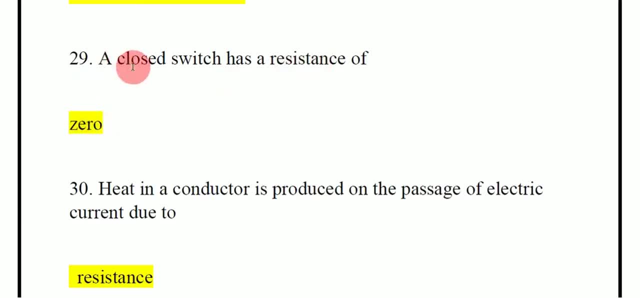 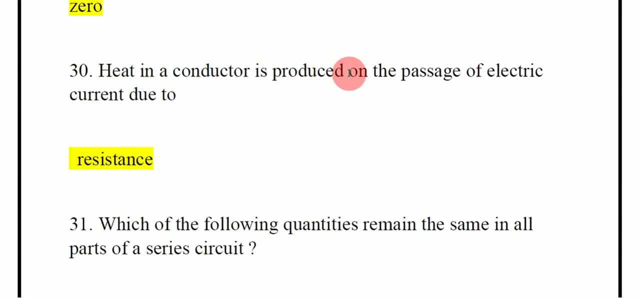 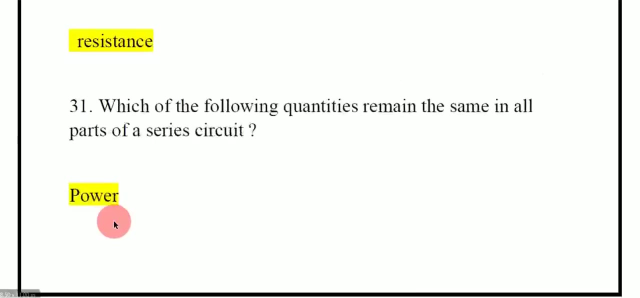 A closed switch has a resistance zero. Closed switch has a resistance zero. Heat in a conductor is a produced on the passage of electric current Due to resistance. so why heat is produced due to resistance? Which of the following quantity remain the same in all parts of series circuit? 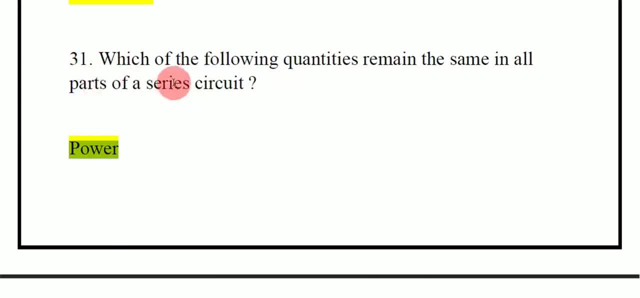 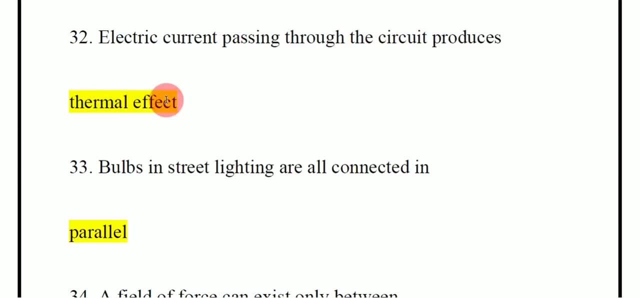 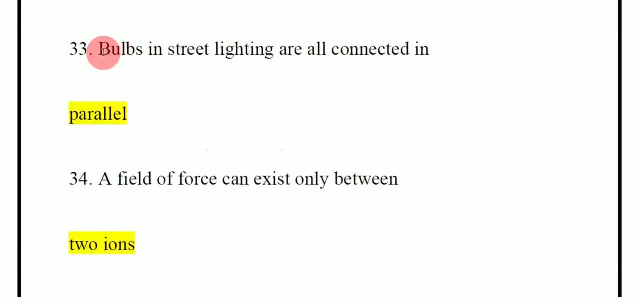 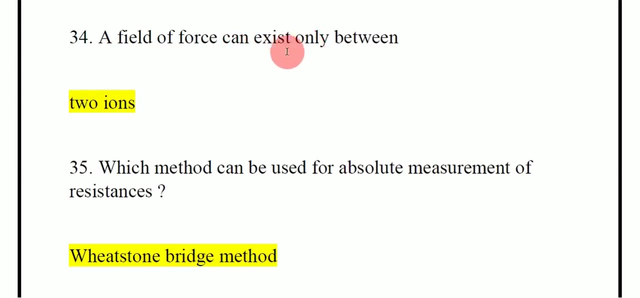 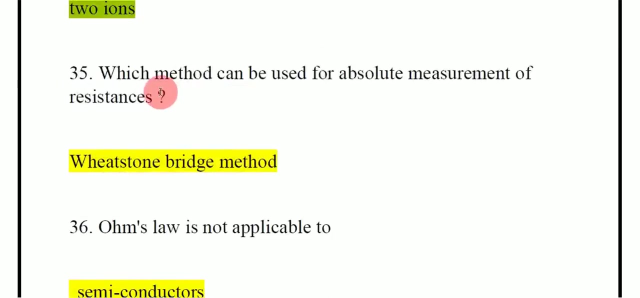 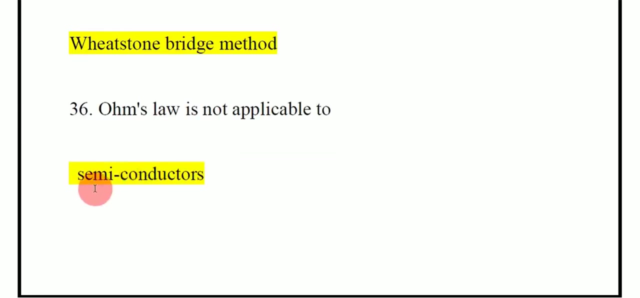 So power power will be same in all part of series circuit. Electric current passing through the circuit produce thermal effect. Okay, when electric current passing through the circuit produce thermal effect, Why, Why, When, When? Whistone bridge method, Ohm's law. Ohm's law is not applicable to semiconductors. 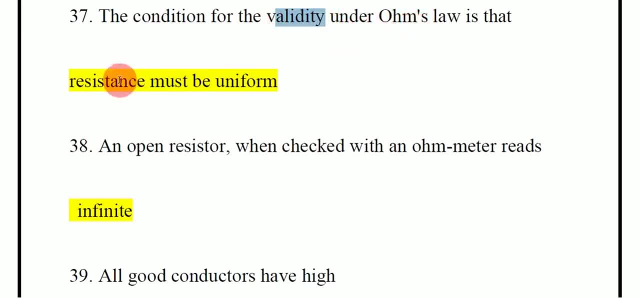 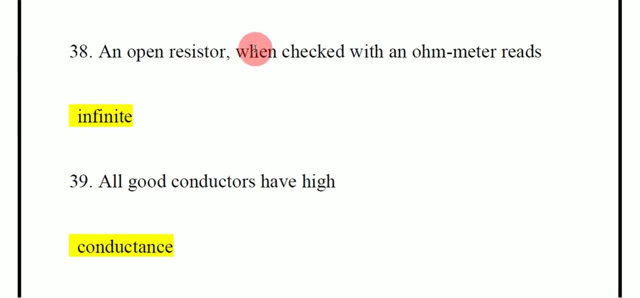 The condition for the validity under Ohm's law. So that validity is: the resistance must be uniform. So this is the condition for the validity under Ohm's law: Resistance must be uniform And open resistors when checked with an ohm meter. 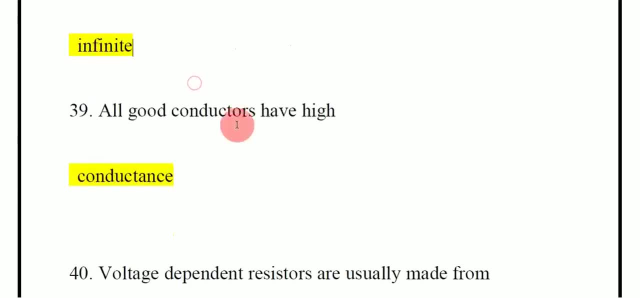 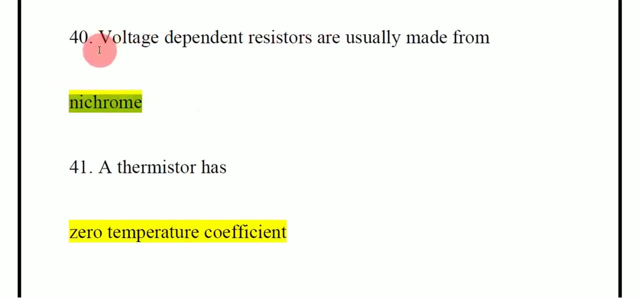 reads infinite. Okay, All good conductors have high conductance. Okay, If good conductors that have high conductance? Voltage dependent resistors are usually made from nichrome. Okay, Voltage dependent resistors are usually made from nichrome- Okay. 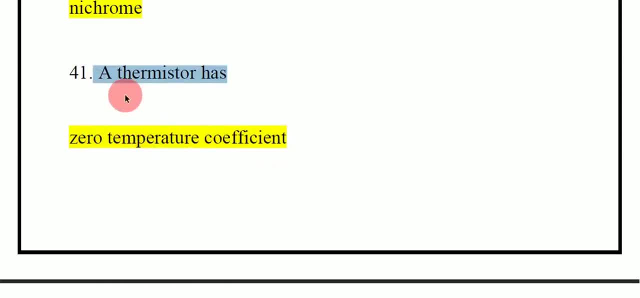 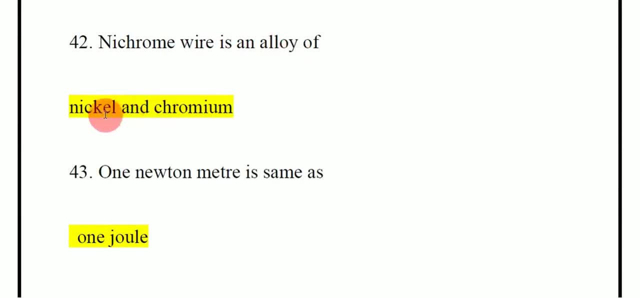 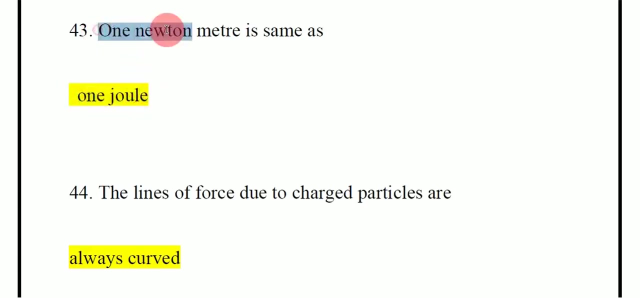 A thermistor has a zero temperature coefficient. Okay, Remember, thermistor has a zero temperature coefficient. Nichrome wire is an alloy of nickel and chromium. Okay, So nichrome, Nichrome wire is an alloy of nickel and chromium. One newton meter is same as one joule. Okay, One newton meter is same as one joule. The line of 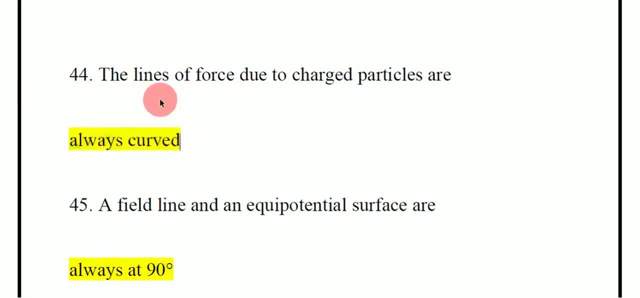 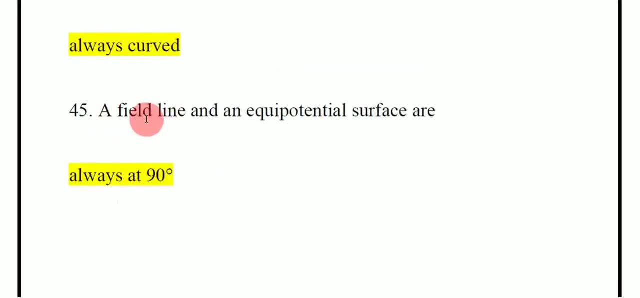 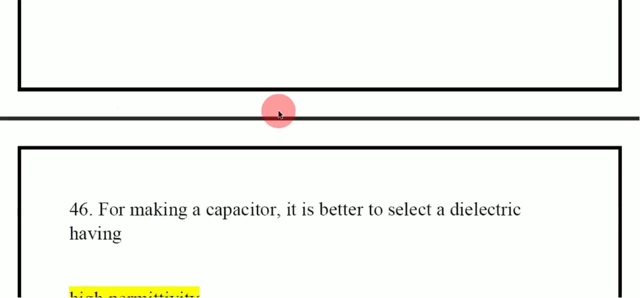 force due to charged particle always curved. Okay, The line of force due to charged particle are always curved. A filled line and an equipotential surface are always at 90 degree. For making a capacitor, it is better to select a dielectric having high permittivity. Okay, If you want to making a capacitor. so these resistors are very good. Anti dimmer One industrial. 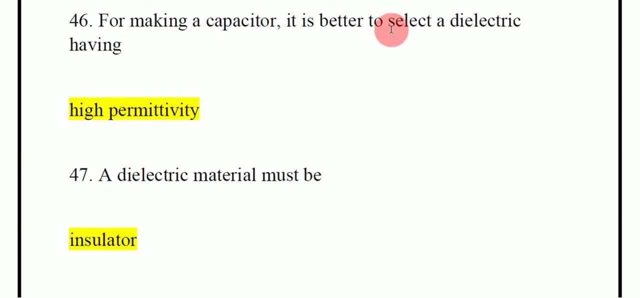 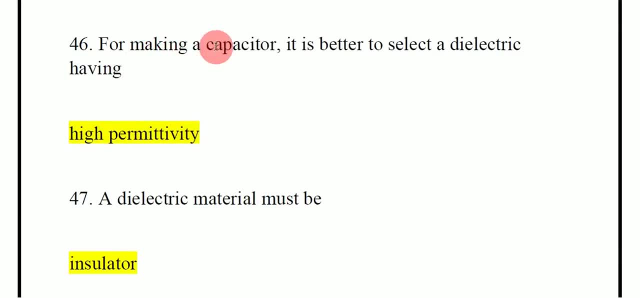 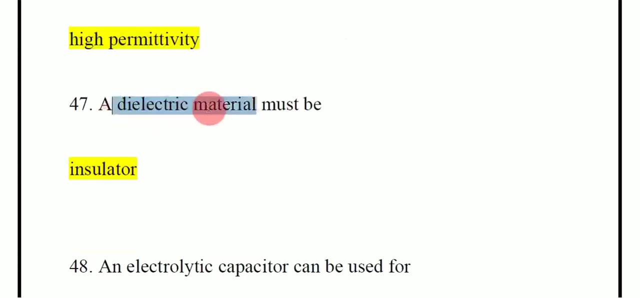 This material demands on: पागे लिंका, सबे जल्क लिंका।. Heavywer notified a. If you want to make a capacitor, So it is better to select dielectric having high permittivity. A dielectric material must be. 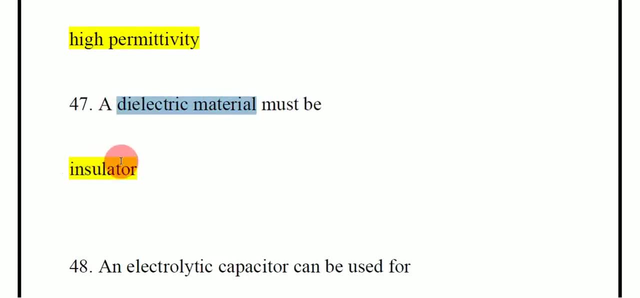 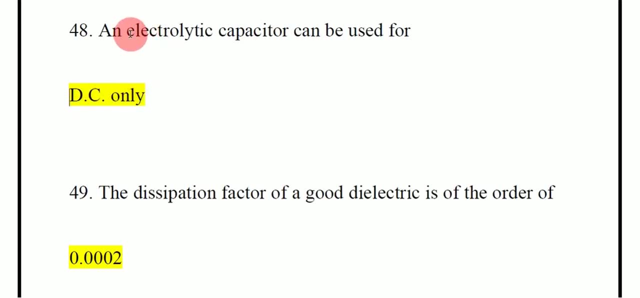 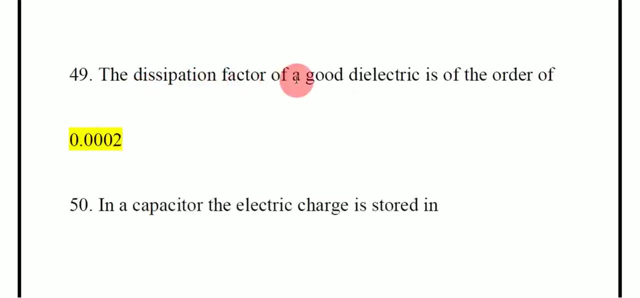 insulator- Okay, dielectric material must be insulator. An electrolytic capacitor can be used for DC only. Remember, electrolytic capacitor can be used for DC only. The dissipation factor of a good dielectric- Okay, dissipation factor for a good dielectric- is of the order of 0.0002.. 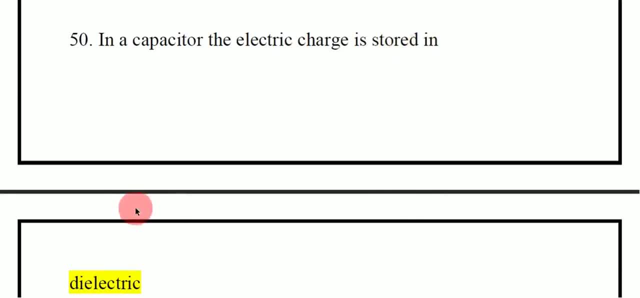 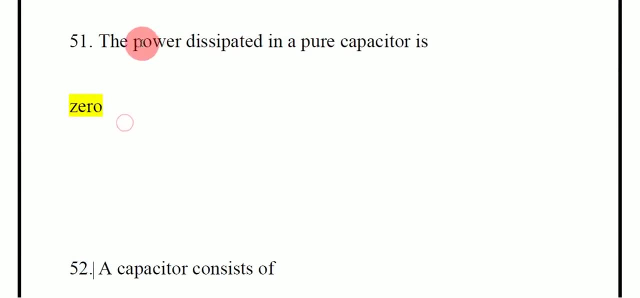 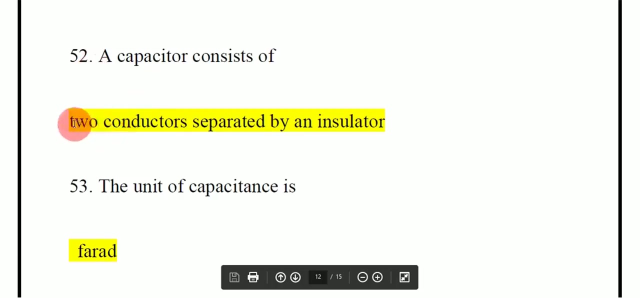 In a capacitor, the electric charge is stored in a dielectric. Okay, so in a capacitor, electric charge is stored in a dielectric. The power dissipated in a pure capacitor is a 0.. Okay, power dissipated in a pure capacitor is the zero. A capacitor consists of two conductors separated by an insulators. 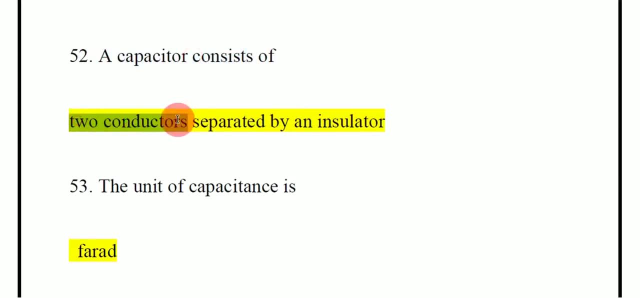 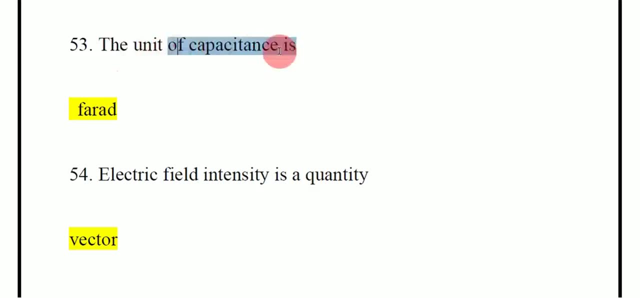 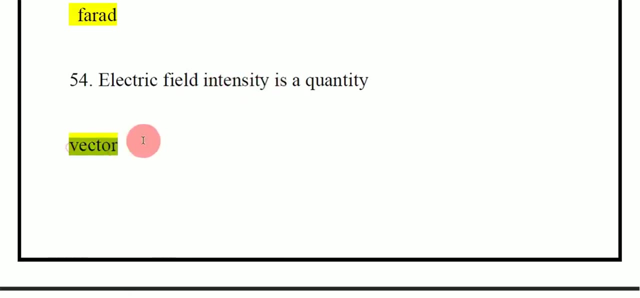 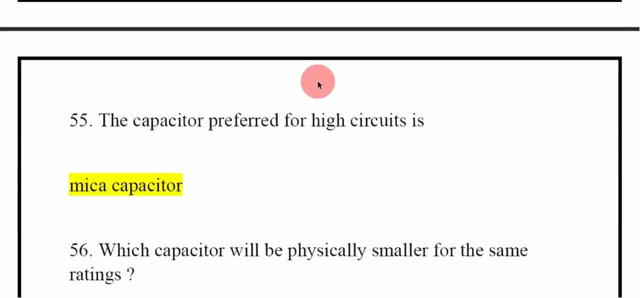 Okay, remember, capacitor consists of two conductors separated by an insulator: The unit of capacitance. the unit of capacitance is the Farad. Electric field intensity is a quantity vector. Okay, electric field intensity is a quantity vector- quantity- Okay, the capacitor. 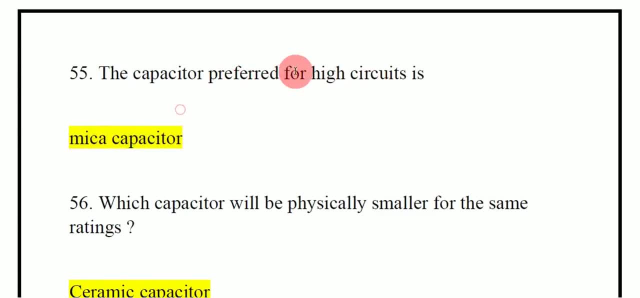 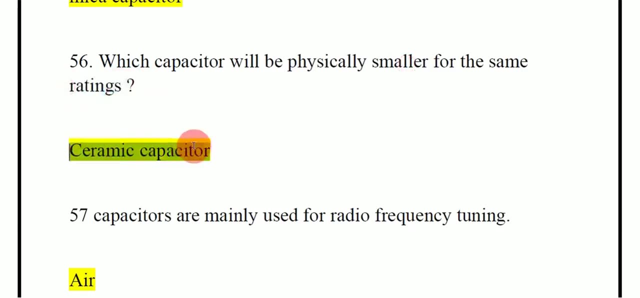 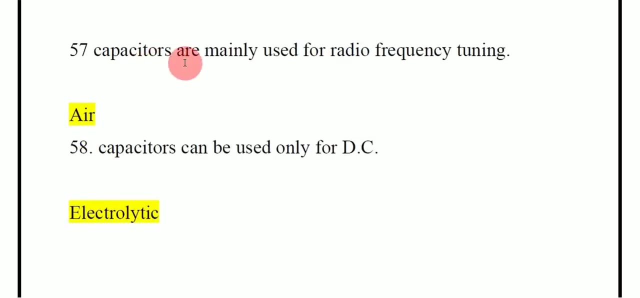 preferred for high circuit is Mica capacitor. Okay, the capacitor preferred for high circuit, high circuit, Mica capacitor. Which capacitor will be physically smaller for the same rating? So, ceramic capacitor, ceramic capacitor is the physically small for the same rating. Capacitors are mainly used for radio frequency tuning. is the 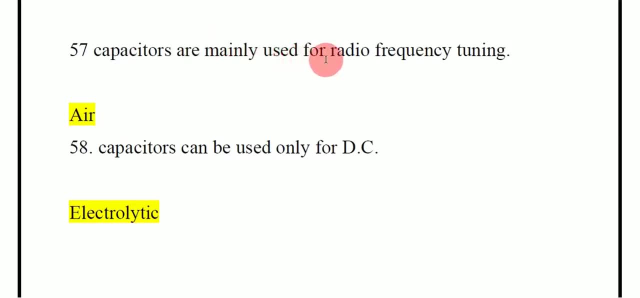 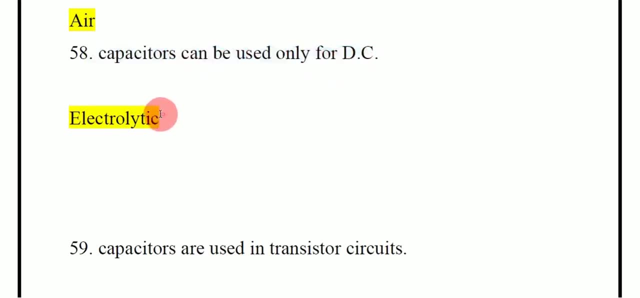 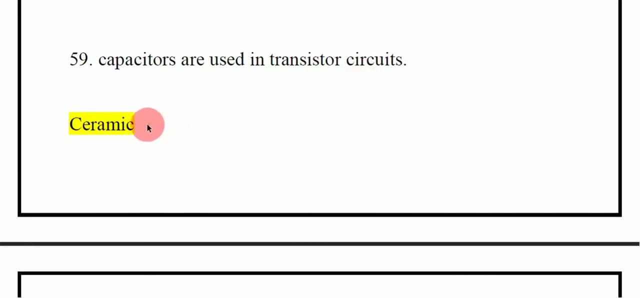 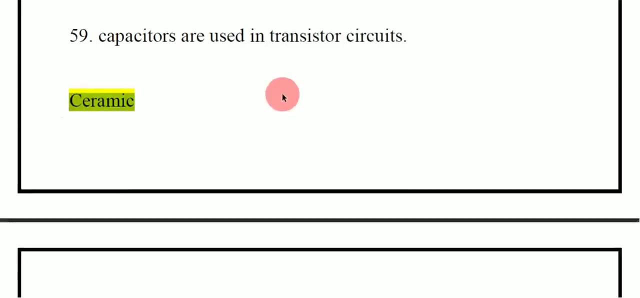 air capacitor. Okay, capacitor are mainly used for radio frequency tuning. is the air capacitors? Capacitors can be used only for DC electrolytic. Okay? capacitors are used in transistor circuit. is the ceramic? Okay? capacitor are used in transistor circuit. is the ceramic capacitors. 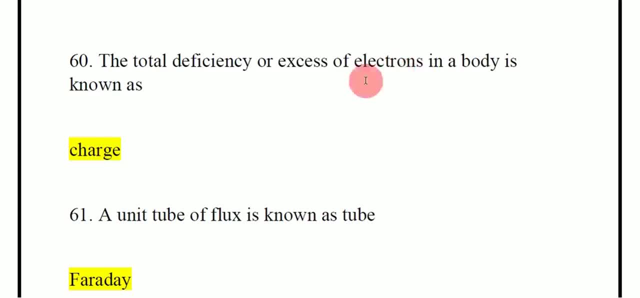 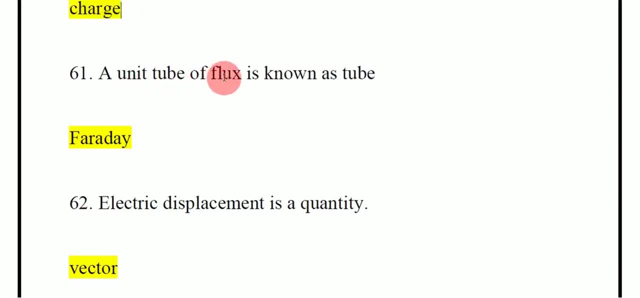 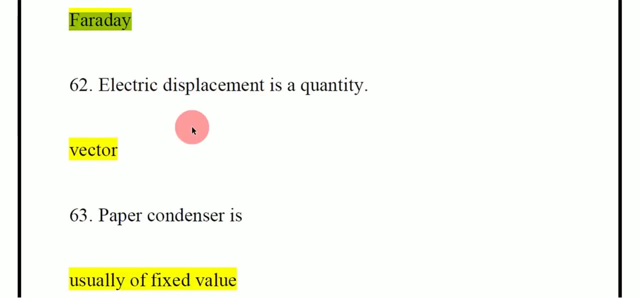 The total deficiency or excess of electrons in a body is known as a charge. Okay, that is known as a charge A unit tube of flux is known as a tube Faraday, Okay, Faraday. Electric displacement is a quantity. is the vector quantity? Electric displacement is a vector quantity. 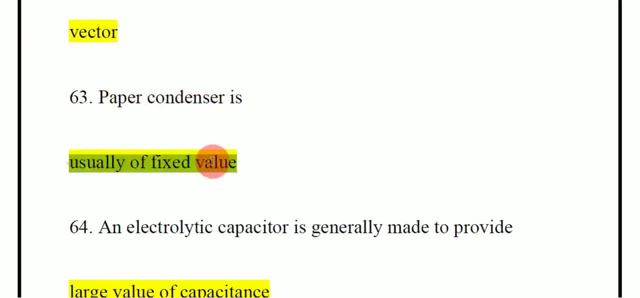 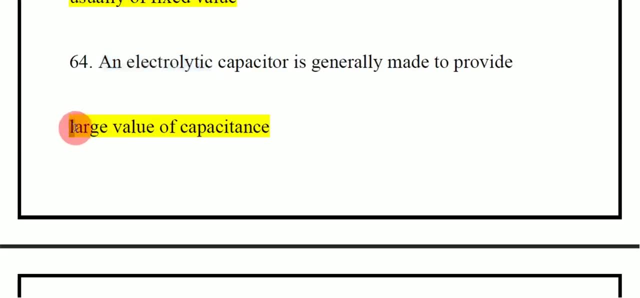 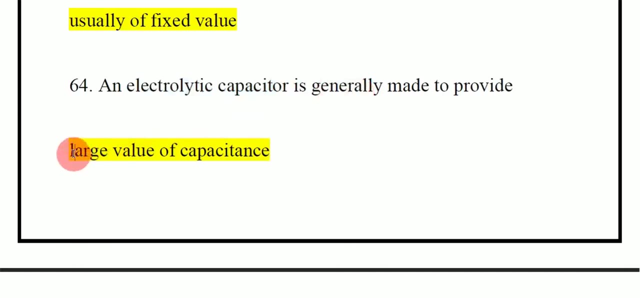 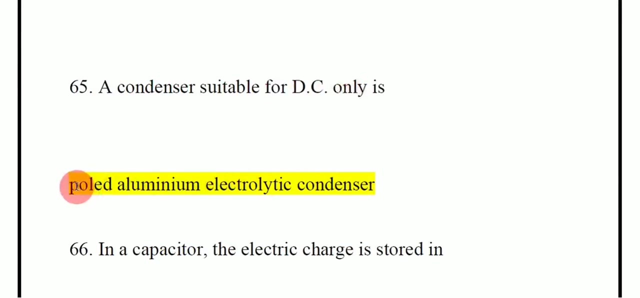 Paper condenser. Paper condenser is usually of fixed value. An electrolytic capacitor is generally made to provide large value of capacitance. Okay, electrolytic capacitors generally made to provide large value of capacitance. A condenser suitable for DC only is polled aluminum electrolytic condenser. So remember. 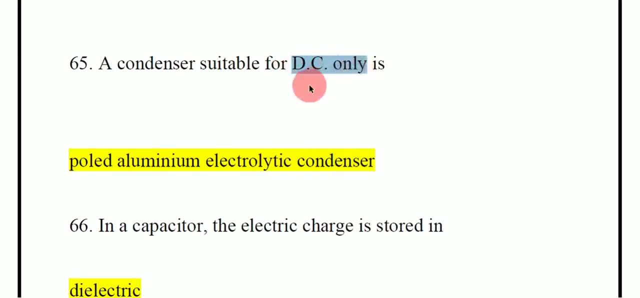 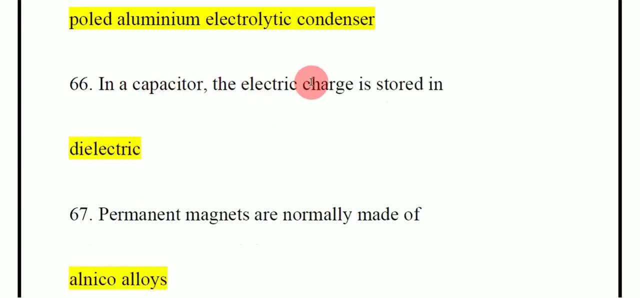 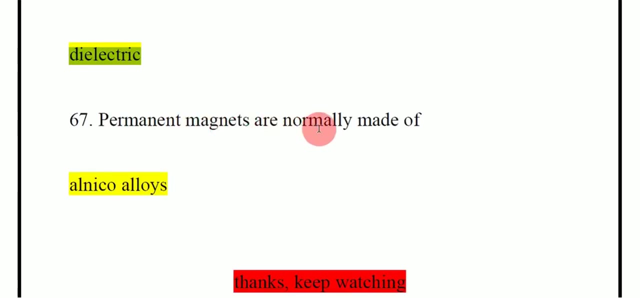 a condenser suitable for DC supply. So DC only, that is polled aluminum electrolytic condenser In a capacitor, the electric charge is stored in a dielectric. Okay, permanent magnet are normally made of alnico alloys. Okay, so permanent magnet. 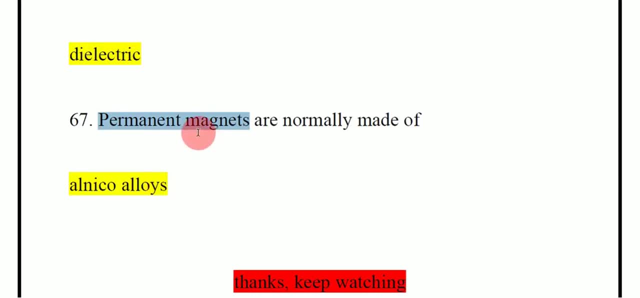 normally made of alnico alloys. So thanks, friends, keep watching and keep learning.